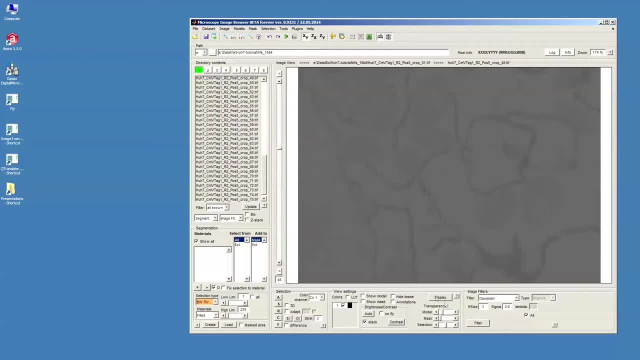 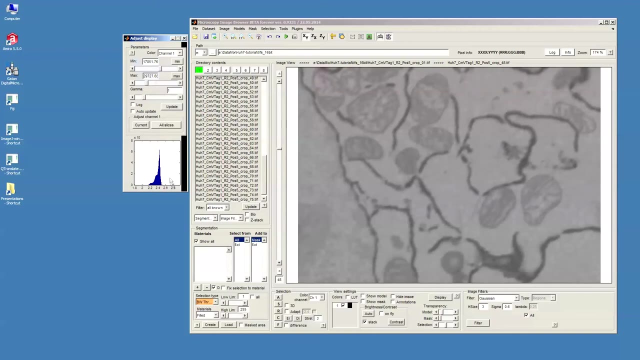 The actual intensities are not stretched through the whole intensity range. In order to stretch the data, we need to press the display button and, using the left key, we can change the left, the minimum value, minimum intensity value- and using the right key, we can change the. 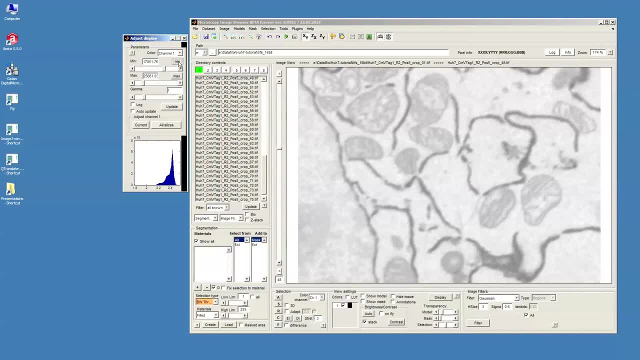 maximum intensity value. Alternatively, we can just click on this min and max button and in this case, the minimum and maximum intensity point for the whole datasets will be found, and then the data will be stretched to this value. What I would like to do, I would like to actually convert the data to 8-bit, because it will decrease. 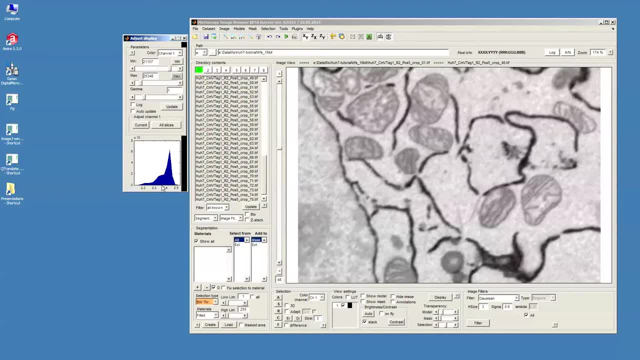 twice the space the data occupies in the memory, and also it will make some of the things much faster. In order to do that, I will actually recalculate the intensities by pressing this all slices- adjust channel. one for all slices button, And what would happen is that the intensity- which is now 21,000, becomes 0, and the intensity which is 25,000, becomes 65,000. 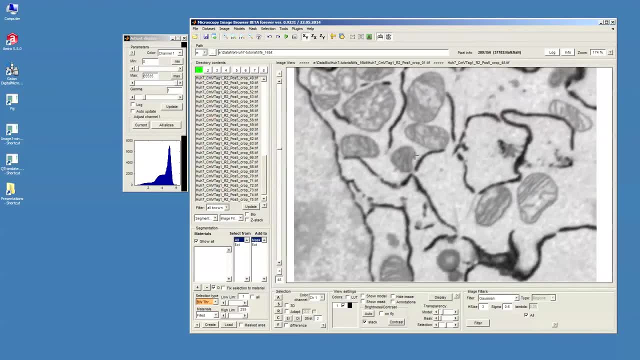 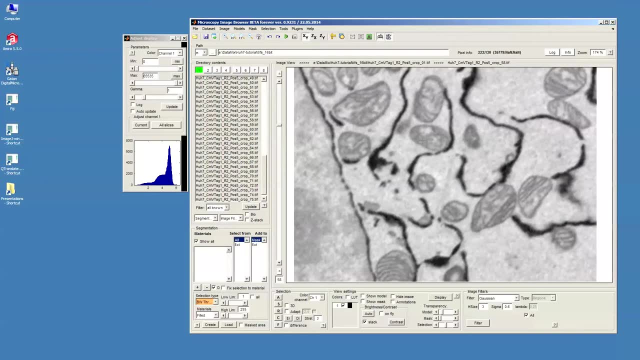 As you can see, now The next step. now the data was stretched, but it's still in the 16-bit format and I need to convert the data to 8-bit format, And this can be done from the menu, image mode 8-bit. 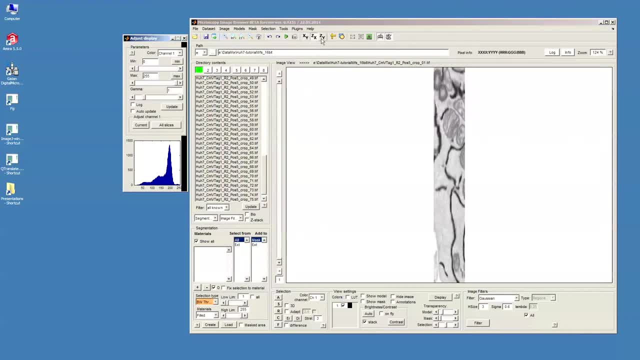 Now the data is converted, We can check the data in the different projections, but actually what you can see here is that the data looks a little bit squeezed, And this is because the actual voxels in this data set are not isotropic, And in order to fix this, we should go to the data set parameters. 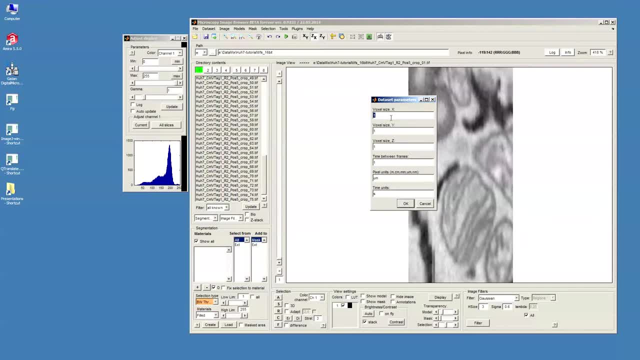 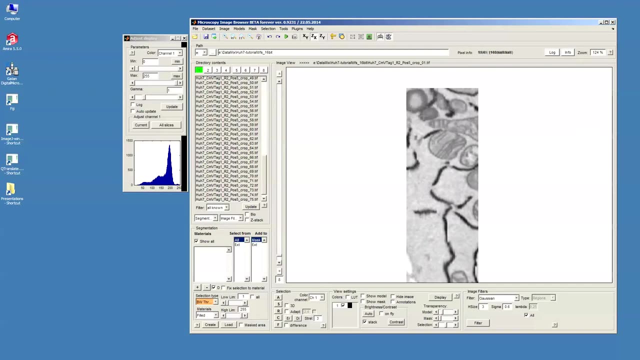 And in here And in here we can define the proper voxel size for this data, And in this particular case I have 30 nanometers XY and 30 nanometers Z resolution. After that you can see that the data was stretched properly and the slippy droplets look quite roundish, as they should be.